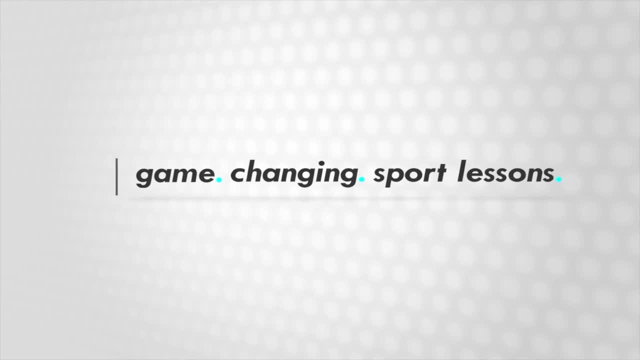 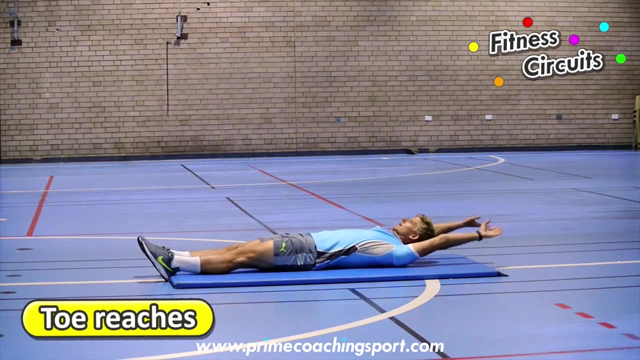 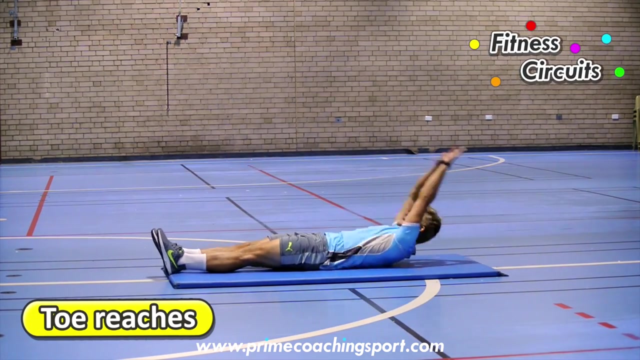 For the toe reaches. you're going to start on the mat lying straight and flat. Once you're straight, you're then going to sit up and reach your toes. That's one. Then you come back down. Two: Stay nice and straight and then touch your toes. Three, Keeping your legs together. 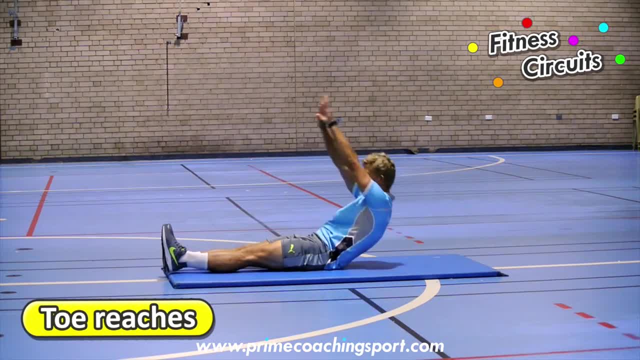 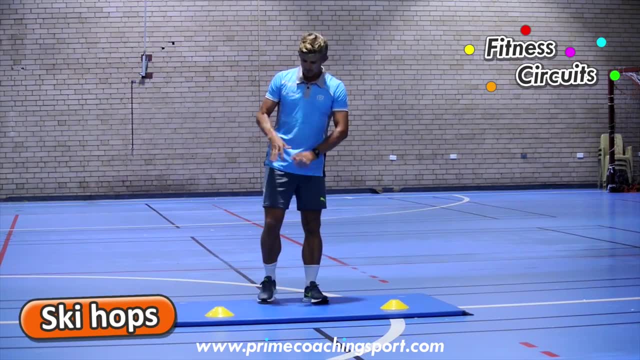 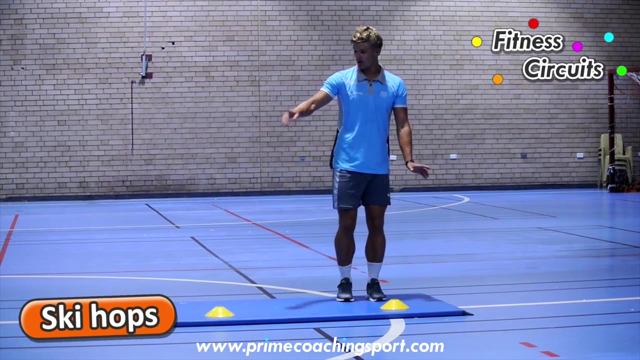 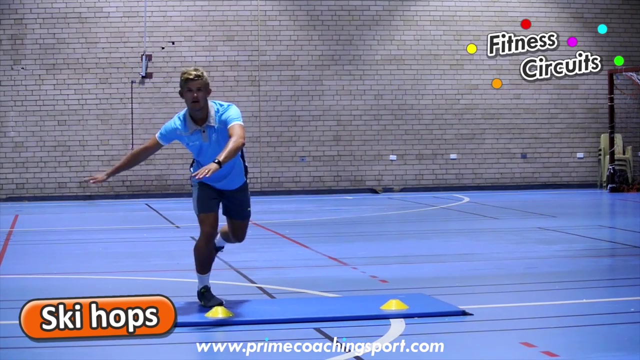 And that's the toe touches, Ski hops. For this one you might have two cones or maybe two spot markers. You're going to start on one cone and you're going to hop over to the other side, balancing on one foot. So I'm here on my left foot, I'm going to hop over and balance on my 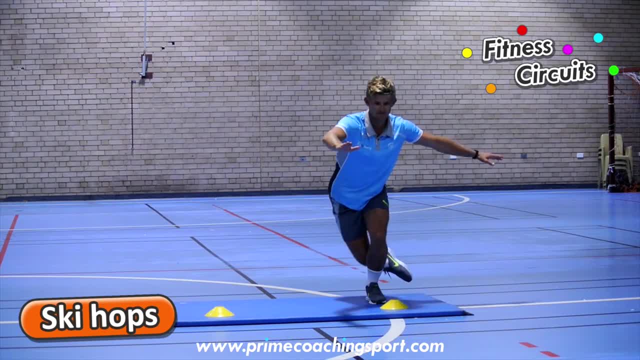 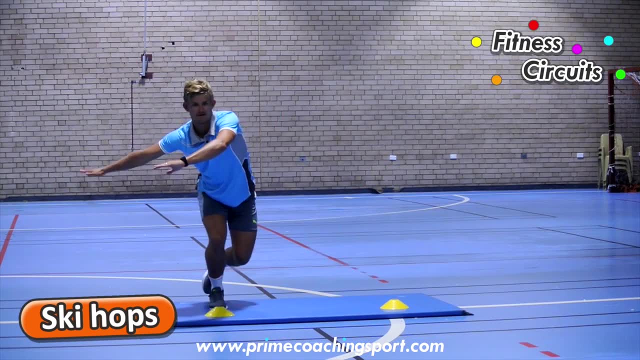 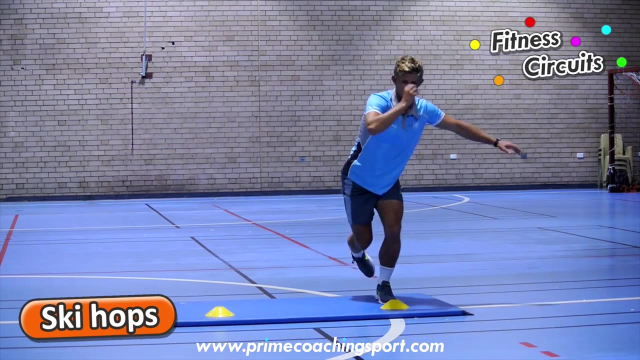 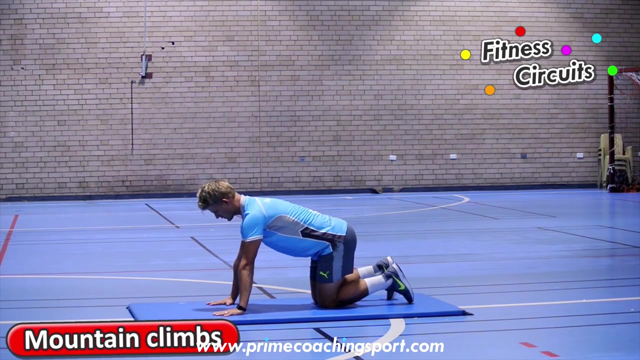 right foot, Hop over to the left and balance on my right foot And right, Keep your arms out to help you balance. So you're always hopping on one foot and that's the ski hops- Mountain climbs. You're going to put two hands- straight hands and straight legs- And now you're. 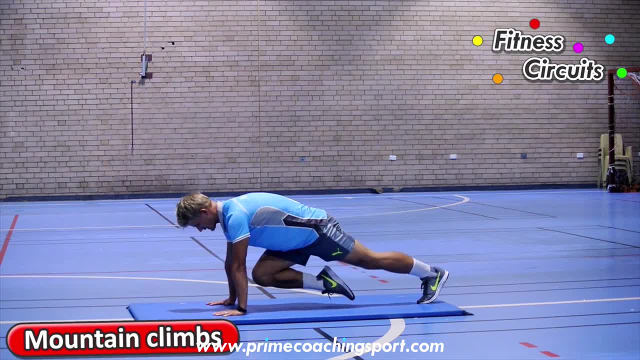 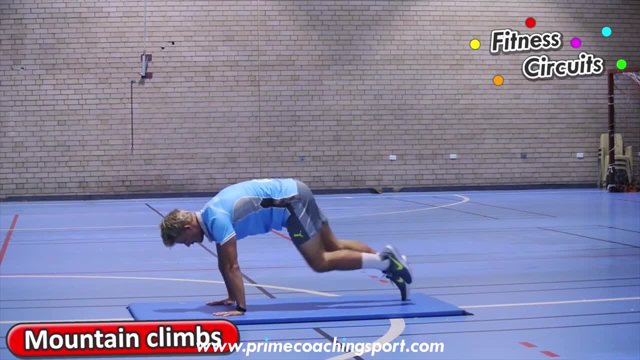 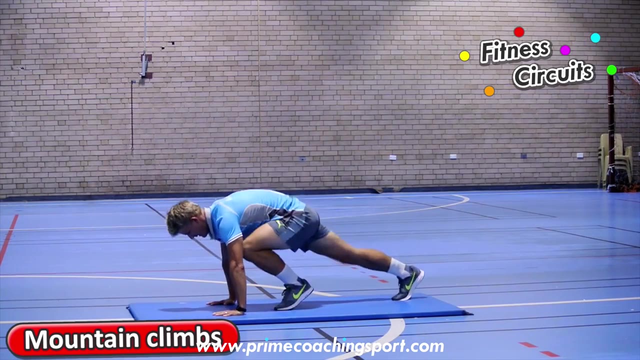 going to lift your knee up and back down and then switch. So my left and right, Keep your back legs straight. So one, two, three, four, five, six, seven, eight, nine. You keep going, and that's the mountain climbs. 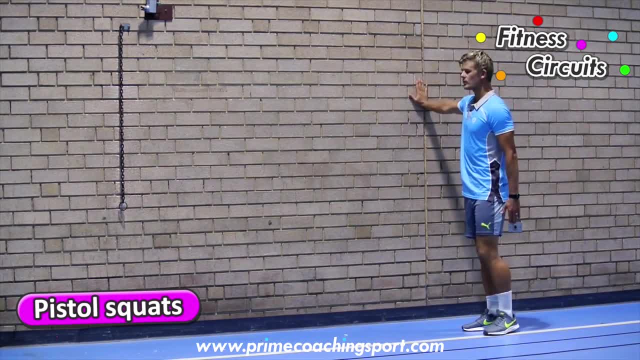 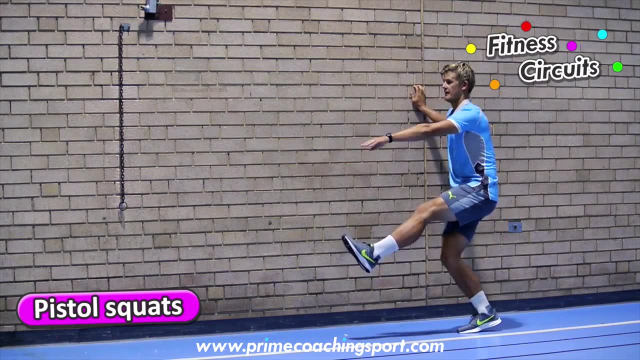 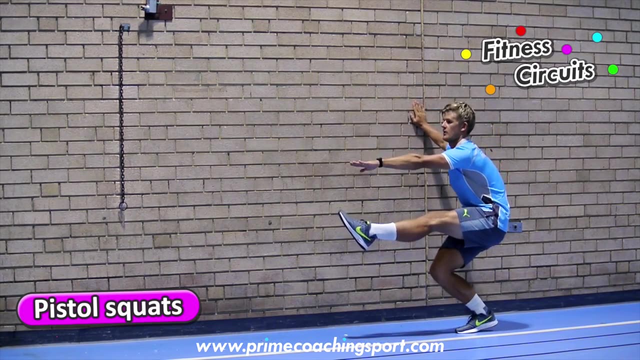 Pistol squats. You're going to put one hand on the wall. You're facing sideways, You're going to put one leg out straight and bend the other and then stand back up. That's one, Two, Three. Try and get your leg out straight. You can use your other leg if you like. 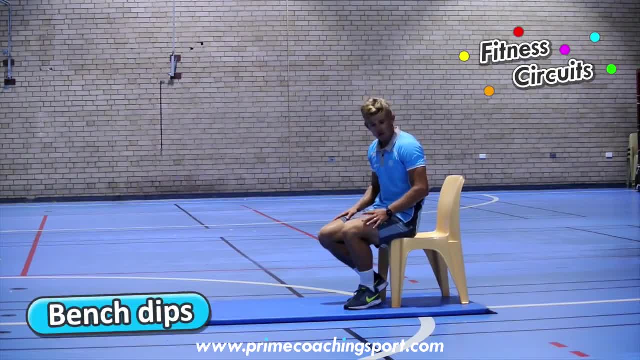 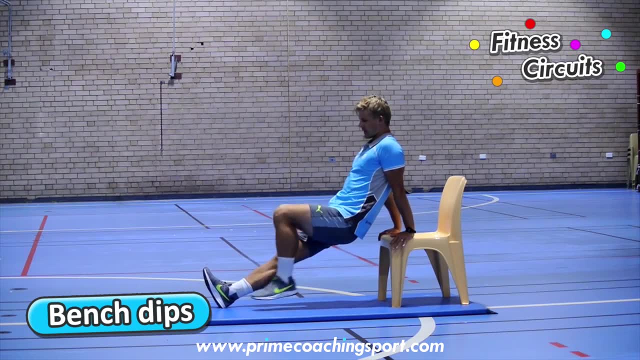 And that's the pistol squats, Bench dips. You might be using a bench or block, or even a chair. What you're going to do? you're going to put your legs out, straightened together in front and your arms behind you here. 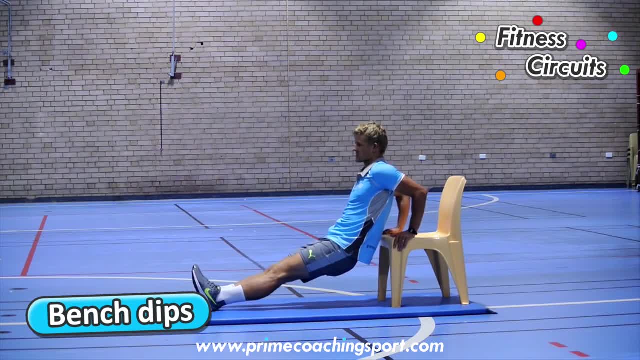 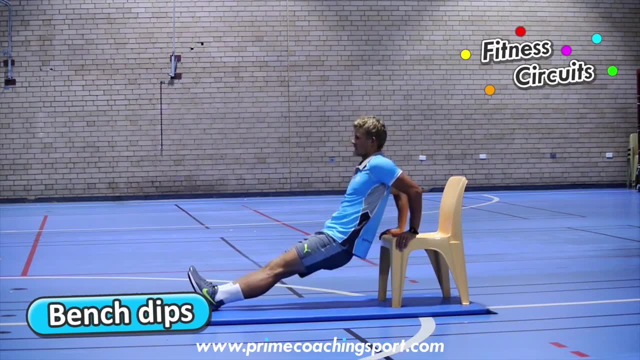 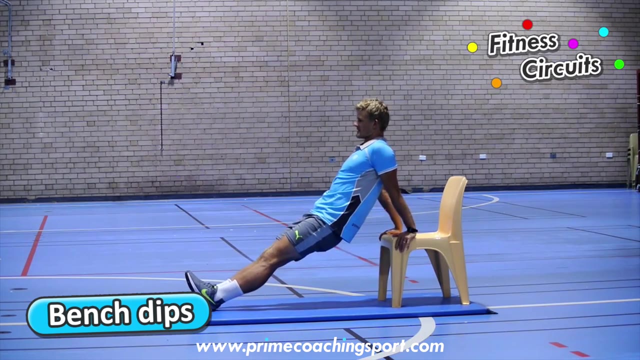 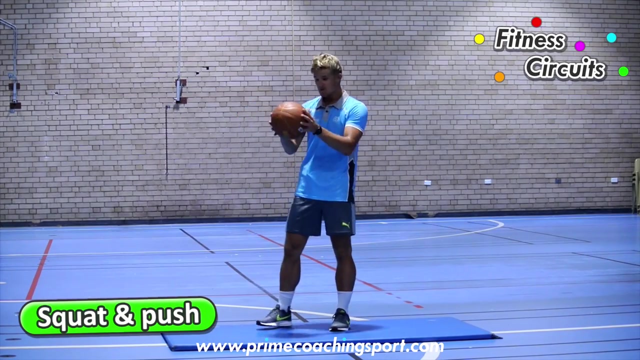 and you'll just get a dip: your bottom below the bench or chair and back up. you see my arms go bent and straight. that's one, two, three, four. make sure you stay nice and straight. and that's the bench dips, squat and push. so for this one with the ball, you've got to hold it in front of you at all times. you're. 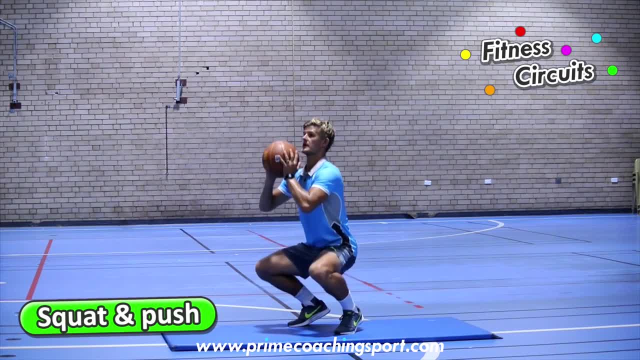 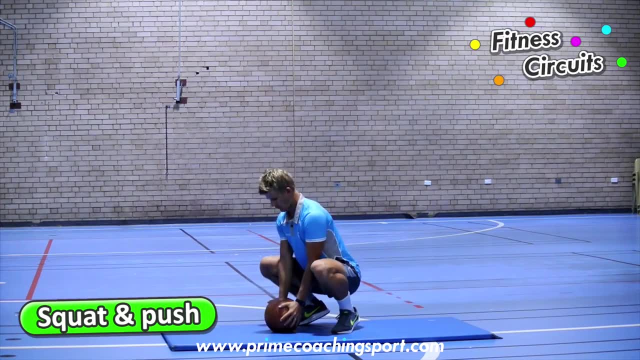 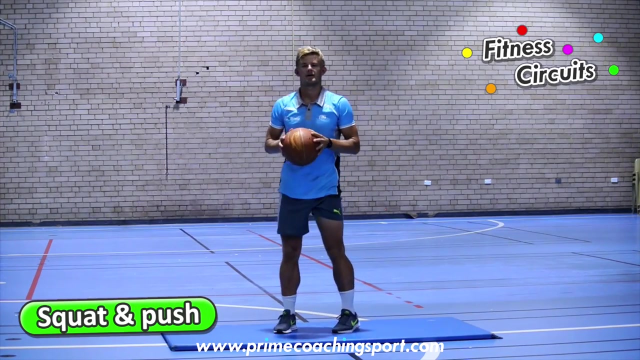 going to bend down, keeping your back straight, and you're then going to reach up and push the ball as high as you can. that's one. so here we go: one, two, three, touch the ball to the ground and then as high as you can, and that's that station. this fitness circuits pack is awesome for any grades. 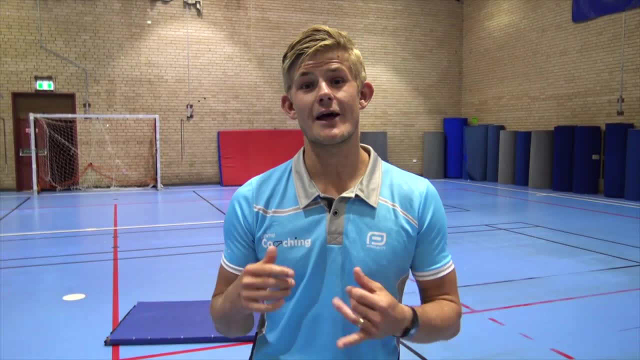 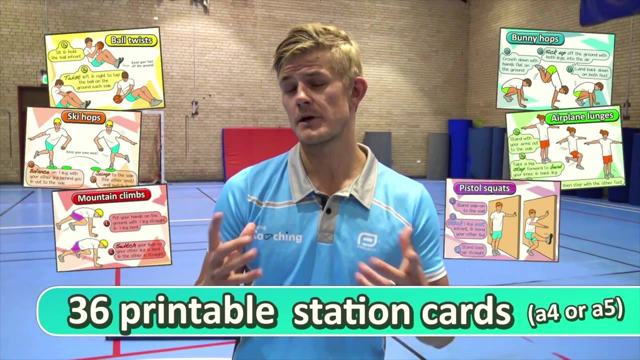 K-12, K-8 teacher. so in this pack you're going to get 36 printable ready to go station cards and you can print them out in A4 or A5 or bigger or smaller, however you like. they're very high quality and they're to be put up around stations. 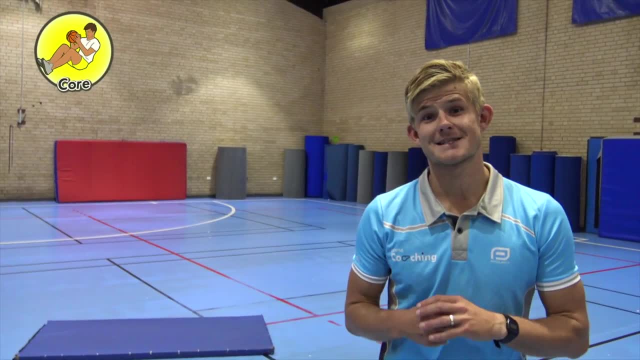 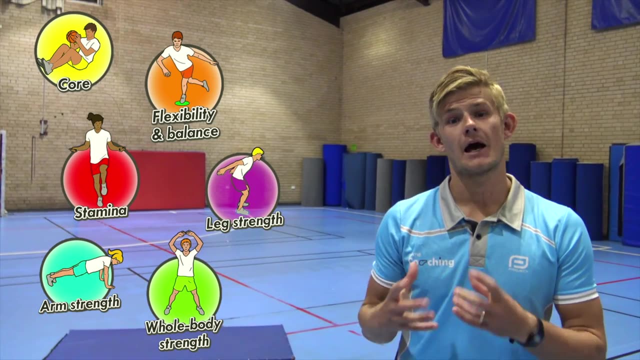 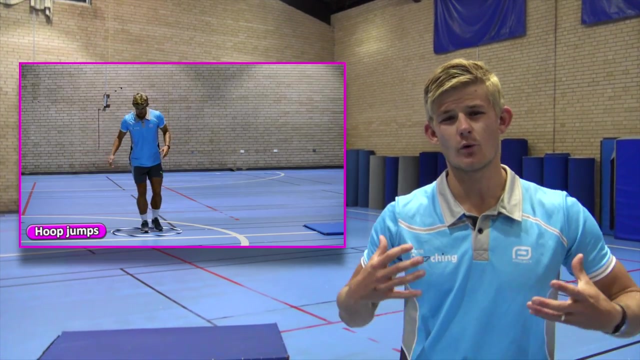 around the sports hall. these dynamic stations cover the six key fitness components. okay, and for each one you're going to have access to online how to perform videos so you can play the stations to your class, so they go out to the sports hall so they know exactly what the fitness. 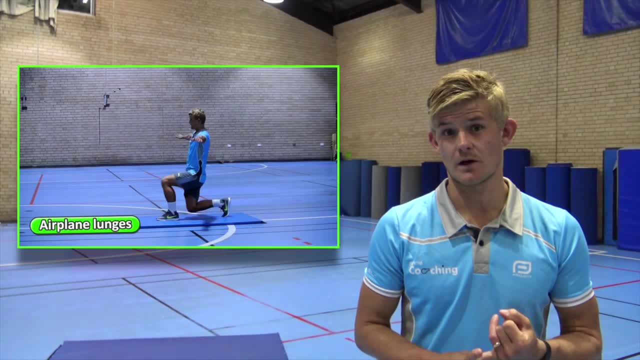 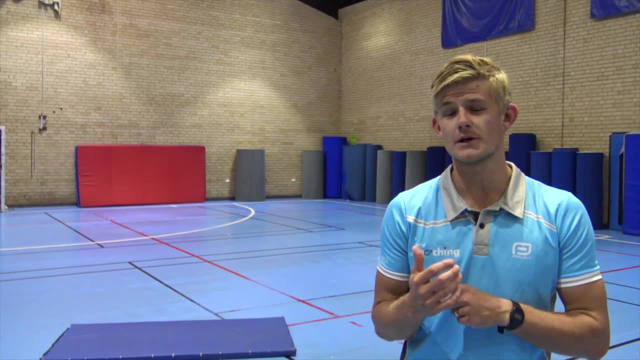 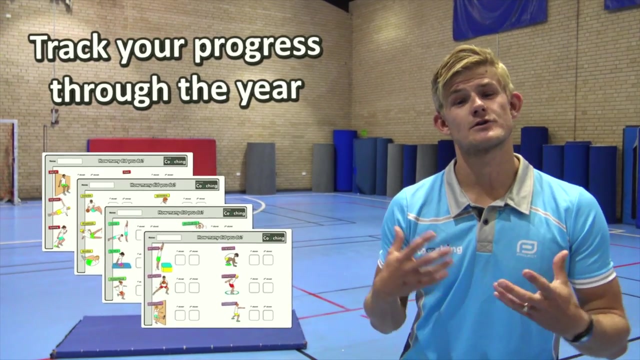 routine looks like, and so they can perform it safely as well. they'll also get testing sheets where students can record their individual scores and their individual points or results, and then- and they'll be able to track their progress as you do it, term by term or even year through year- they can track. 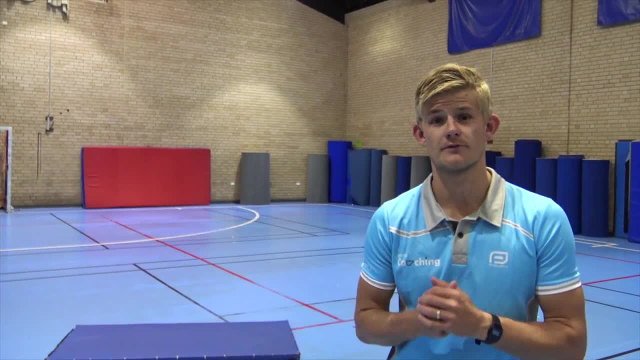 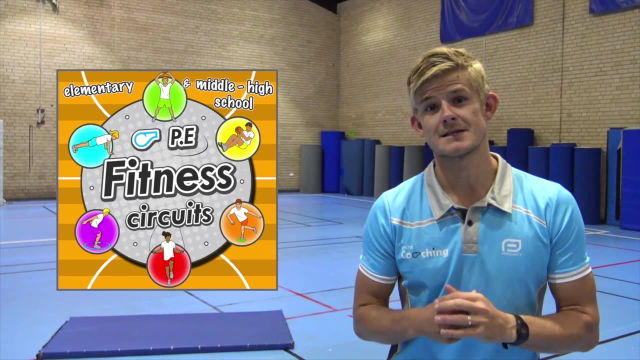 their fitness results and see how well they do and see how well they can improve. so if you're looking for some exciting dynamic setup and follow station cards, make sure you check these out.